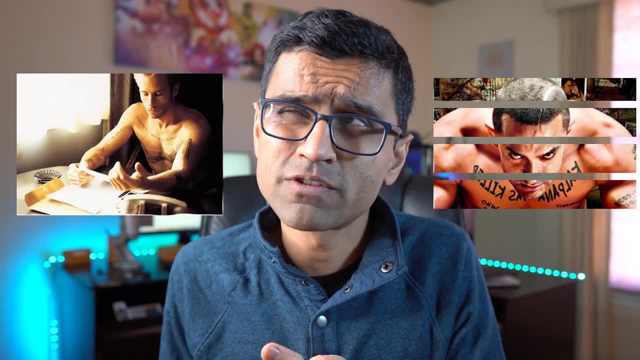 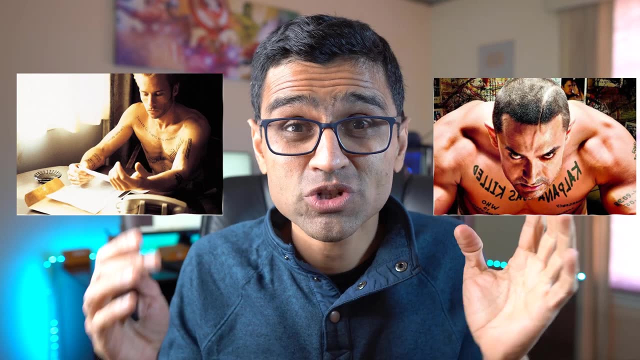 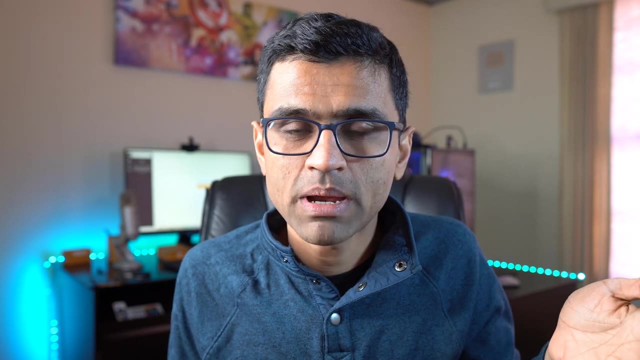 Have you seen this movie called Memento? or there is a Bollywood movie called Ghazni. Our basic RNNs are like the heroes of that movie. They suffer from a short-term memory problem. LSTM is a special version of RNN which solves this short-term memory problem, and in this video I will explain LSTM in a very simple manner, using real-life examples. 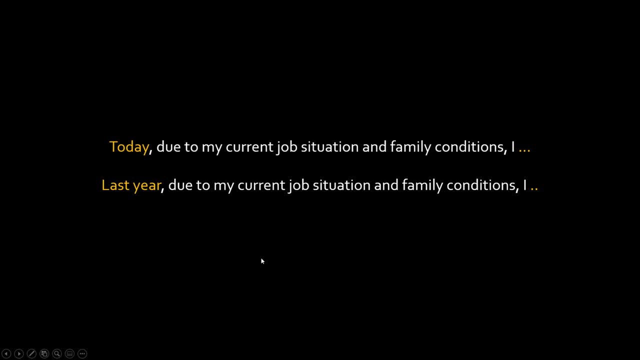 Let's say you have NLP task for sentence completion Here. in both the sentences, based on what word appeared in the beginning, your autocomplete sentence might be different. For example, for the first one I would say I need to take a loan, whereas for the second one I would say I had to take a loan. and this decision between need and had was made based on what appeared at the very beginning. 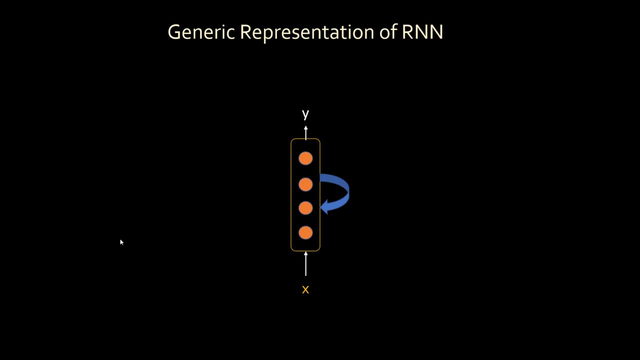 Now looking at our traditional RNN architecture. if you have seen my previous videos, you would know this is how RNN architecture looks like. So if you have not seen those videos, I highly recommend you watch them, because they are kind of a prerequisite. 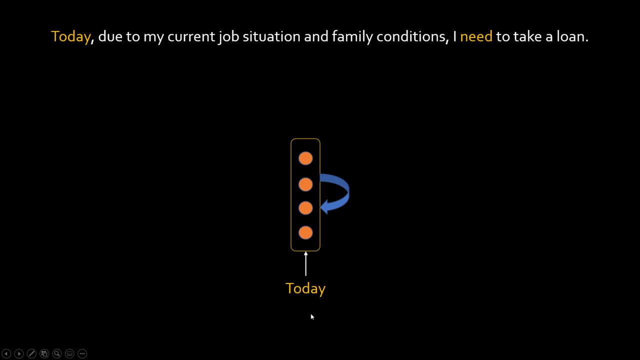 Here when you feed the sentence word by word. so first you will feed, today it will learn some weights. there is an activation which is fed back. Now you work on the second word which is due, then the third word which is to. 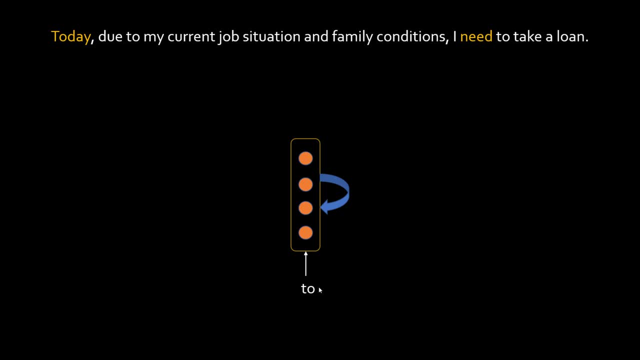 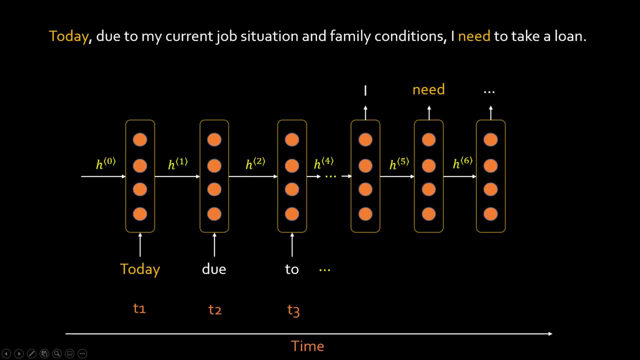 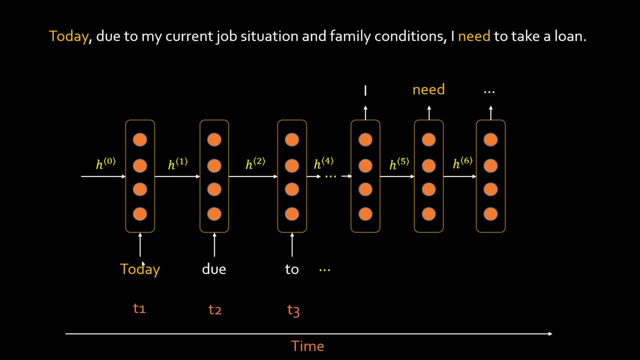 this word need. it needs to know about the word today which appeared at the very beginning of the sentence. and, because of vanishing gradient problem, the traditional RNNs have short-term memory so they don't remember what appeared in the beginning of the sentence. they have a very short-term. 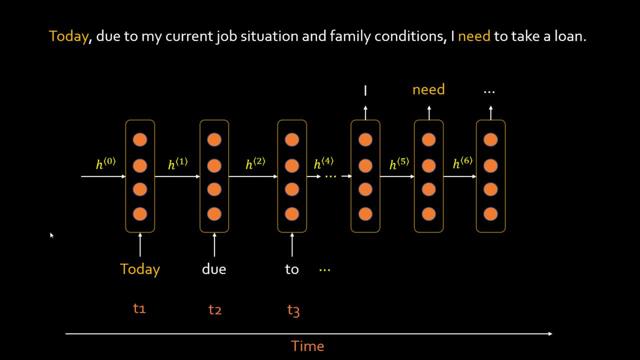 memory of just few words which are like nearby. hence, to auto complete this kind of sentence, RNN won't be able to do a good job. similarly, this is the second sentence. you know where head was derived based on the earlier word, which is last year. now let's look at the network layer a little more in detail. so I'm going to 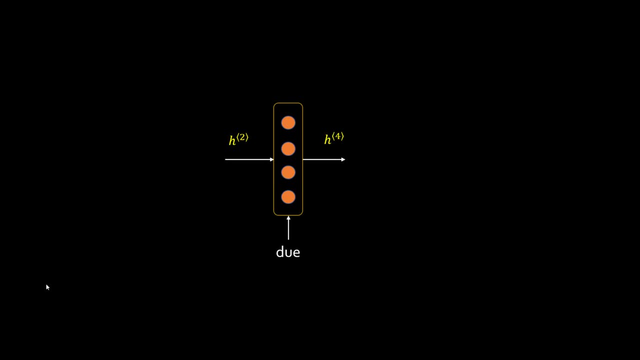 just expand this particular network layer which looks like this. so there are set of neurons in that layer and this hidden state is nothing but a short-term memory. okay, so I'm just going to remove this neurons, just to kind of make it simple. and this square box is called a memory cell because this hidden state is actually containing the. 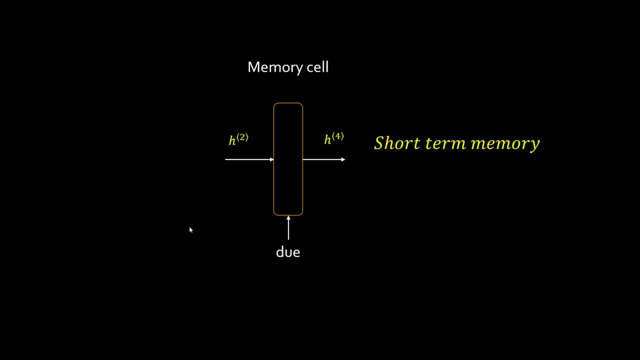 short-term memory. now, if you want to remember long-term memory, we need to introduce another state called a long-term memory. so that state is called C. so there are two states now: hidden state, which is short-term memory, and there is a self state which is a long-term memory, and we will look into this in detail. how exactly. 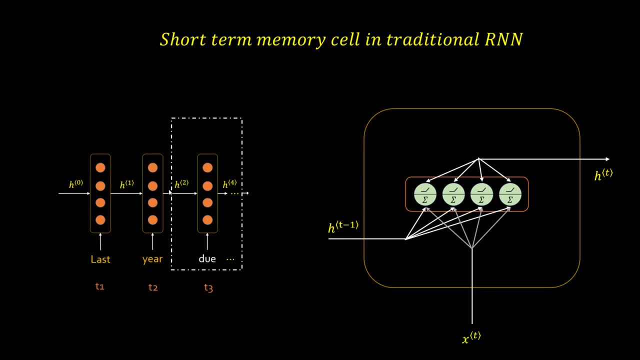 this will work. but going back to our short-term memory cell in traditional RNN, if it looks something like this: so I have drawn the vertical neurons here, but you can draw them this in a horizontal fashion as well. so it's just a layer of neurons and your XT and HT are vectors. so when you have a word, 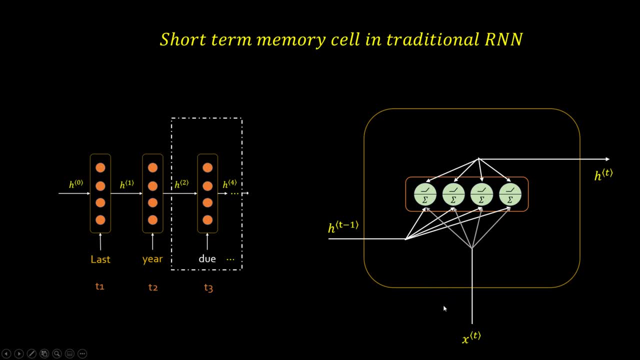 for example, you will first convert into a vector- vector is nothing but a list, list of numbers- and your hidden state will be also a vector. and using both these vectors, you will do, you know, like Sigma operation, like weighted multiplication, and then you apply activation function, which is which is 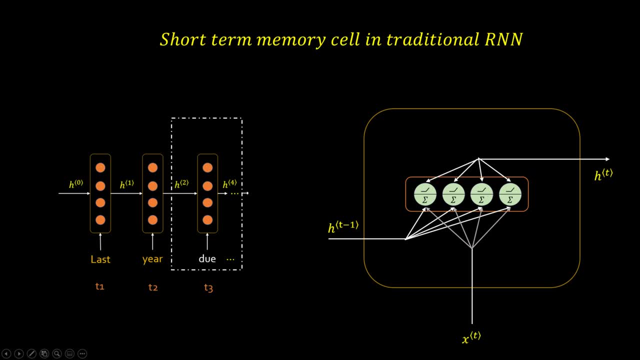 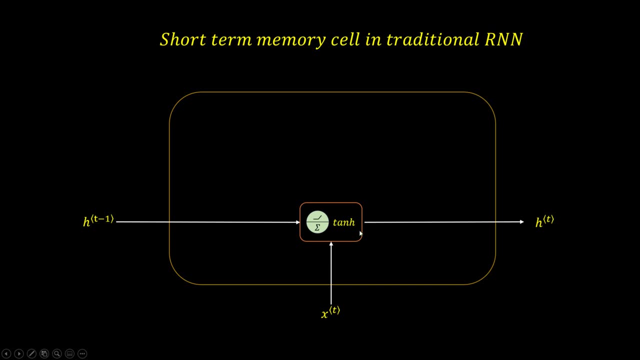 tanh in the case of RNN, and then you get a new hidden state. so here is a simplistic example, right? so here you have tanh, you have weighted sum going on, and this is how the short-term memory cell looks in traditional RNN. in LSTM we are going to introduce a new cell state for a 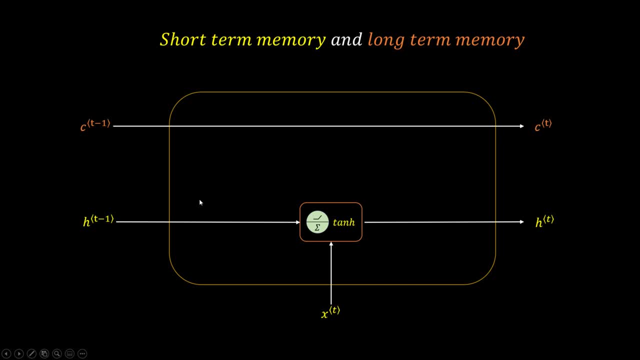 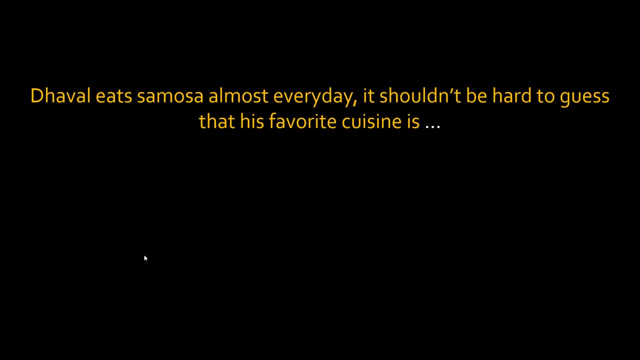 long-term memory. so let's say, there is this cell state. okay, now let's see how exactly this works by looking at one more example. I love eating samosa, by the way, so I have one more sentence for you to auto complete. can you tell me what? 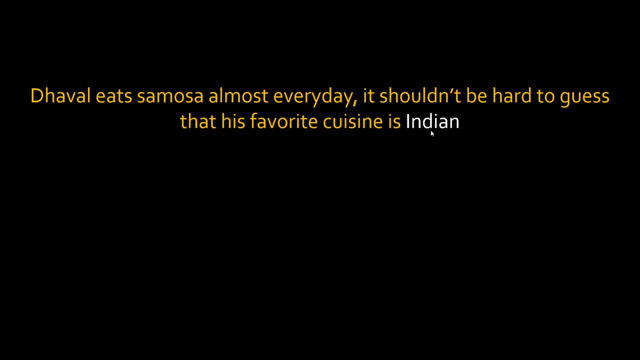 would you put here at dot dot dot. well, obviously, Indian samosa is an Indian cuisine. so you will say his favorite cuisine is Indian. now take a pause and think about this. when, as a human, when you make this guess, when you are processing this sentence, which words? 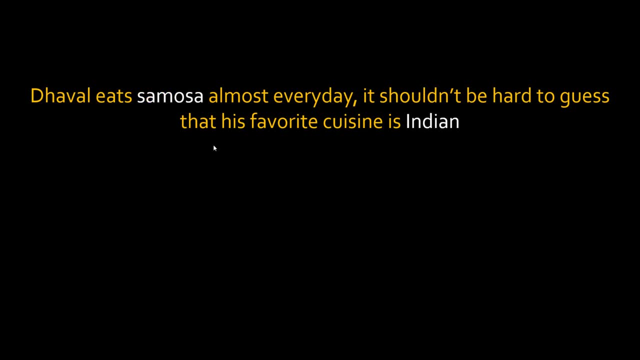 told you that this will be an Indian cuisine. well, it is this word, samosa. if I didn't have samosa here, if I had just had eat or everyday eat. so based on these words, you can't guess it is an Indian cuisine. right, there is some keywords. if you are doing a movie review, for example, you're looking 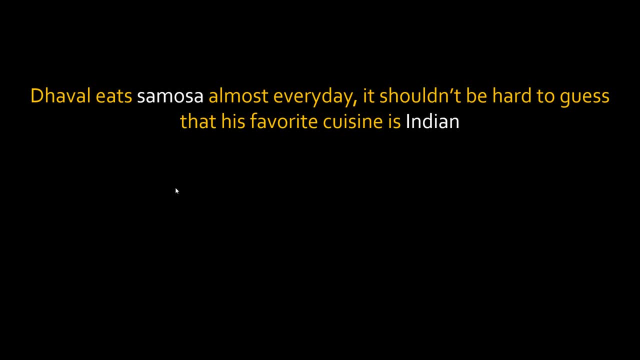 for keywords like okay, excellent or, you know, terrible movie or amazing, the hero performed very well. so you're just looking for specific words and the remaining words you can actually ignore. now let's see how our traditional RNN would behave for this sentence. so our traditional RNN would behave for this sentence. so our traditional RNN would behave for this sentence. so our 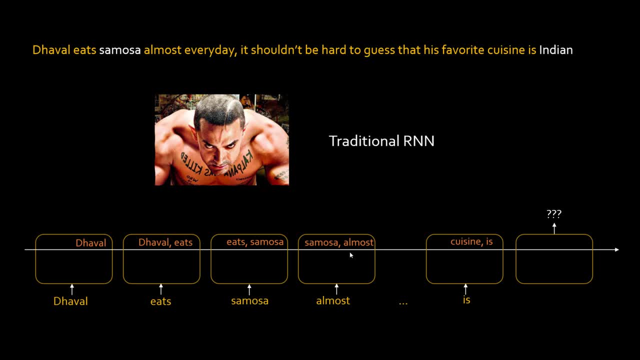 traditional RNN, which is like Amih Khanimage, coffee sne, having short-term memory. when you feed all these words, it can remember only, let's say, last 2 words. in reality RNN's can remember more words, but I'm just giving a simple example, you know, just to explain this concept. so let's say they have. 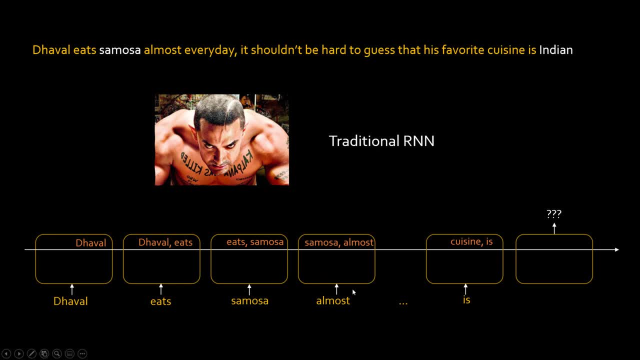 short-term memory, just remember only 2 words. so when you are at this sentence, almost, for example, it remembers almost and the Samosa, like the two words last words here: cuisine, is, it will remember is and cuisine. so at this point it doesn't have knowledge of samosa. so then, for a traditional RNN it is hard to make a 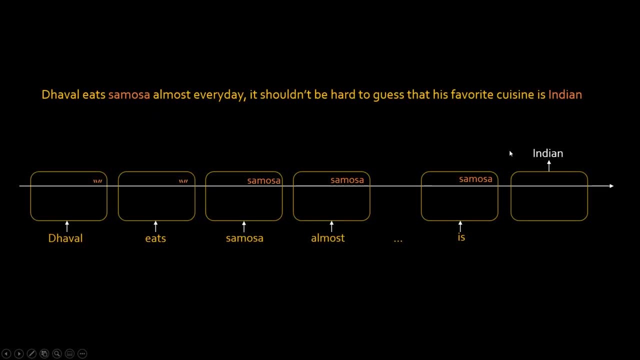 guess that the cuisine is Indian. what if we build this long-term memory, along with short-term memory, in such a way that we store the meaningful words or the key words into this long-term memory? so when I feed the world or eats, it will not store it. this is a blank string. it will not store it in a long-term memory. 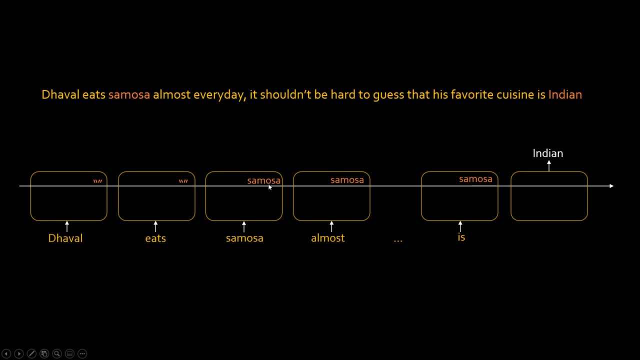 but when you find things like samosa, it will store it in a long-term memory. see, samosa when you get almost almost is also not important, so I just store samosa here and when I go all the way here now when I have to make a 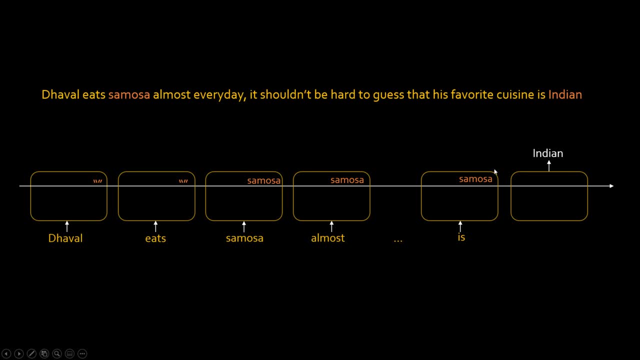 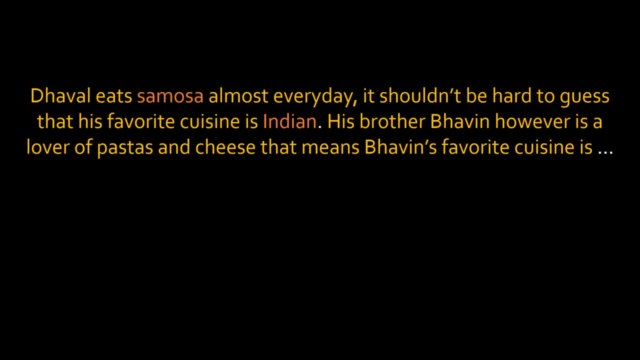 prediction on cuisine and I have that memory that this we are going to make a prediction on cuisine, and I have that memory that this we are talking about samosa and hence it has to be Indian. let's look at little more complicated example here. while I love Indian cuisine, my brother Bavin loves 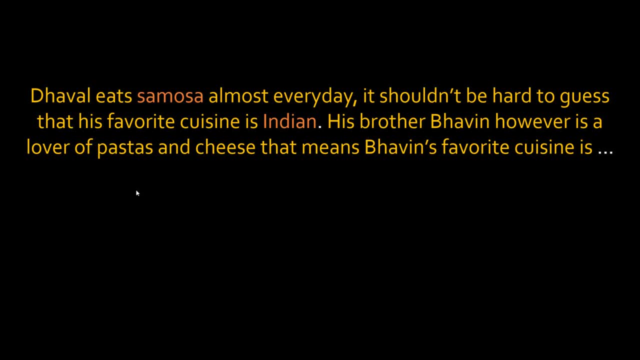 which cuisine? do you have any guess? if you read the sentence carefully, you will figure it is an Italian cuisine, and you made that decision based on the two keywords, which were pastas and cheese. so again, you are reading the sentence and you are keeping the same sentence, and you are keeping the same sentence, and 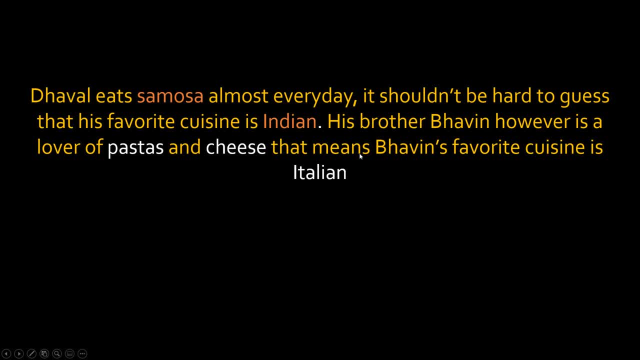 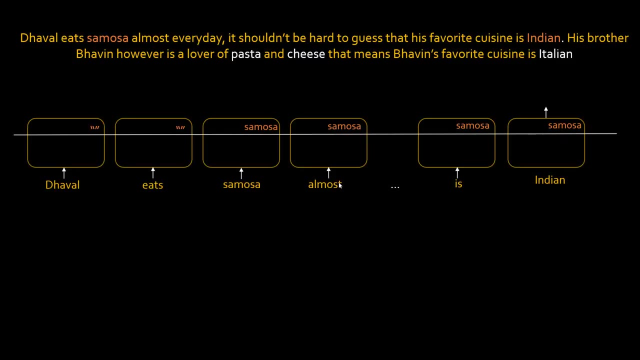 you are keeping some keywords in memory and throwing everything out like and that means these are not important. for you. the important key words are pastas and cheese. based on that, you make a decision that it is an Italian cuisine. so, going back to our RNN with 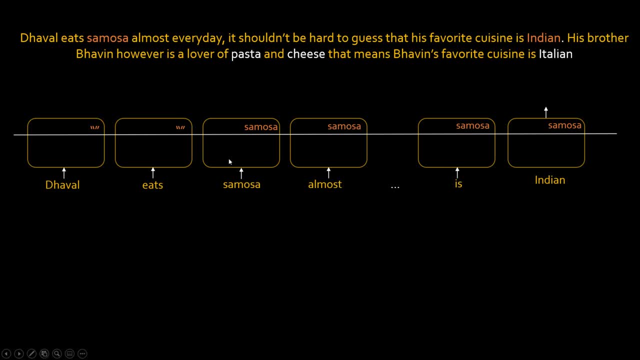 long term memory. when you encounter, let's say, samosa I, you will store samosa in your long term memory, but you will keep on storing samosa until and you encounter pasta. so now, the moment you encounter pasta, you need to forget the previous long-term memory, which is samosa. so here I threw that thing out. 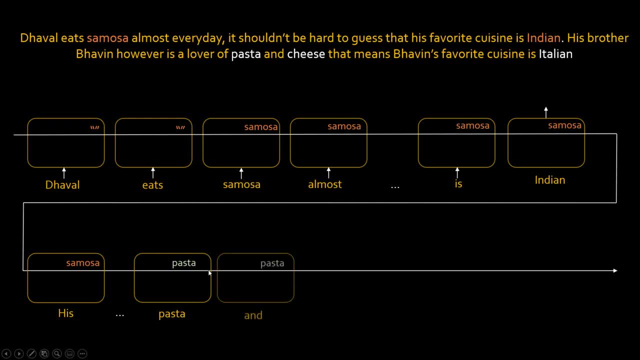 and I have new memory, which is pasta, and then you keep on preserving this until you hit cheese. so when you hit cheese, you need to add that. so now you can't ignore pasta, you need to add cheese on top of it and then in the end, when you 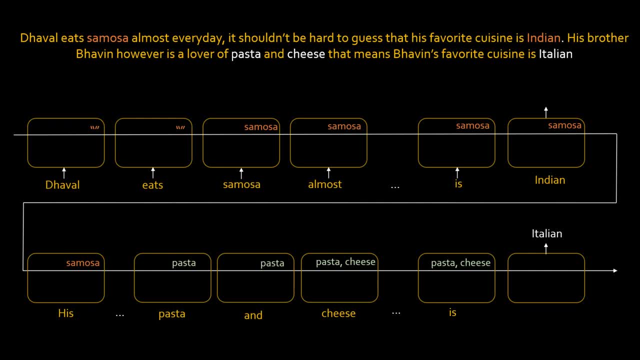 are about to be asked. you know what is your answer for autocomplete. you will say Italian, because you have the memory of pasta and cheese. now you would ask me: how do you make this decision? how do you, let's say, when cheese comes, you don't discard pasta, but when pasta comes, you discard samosa. well, 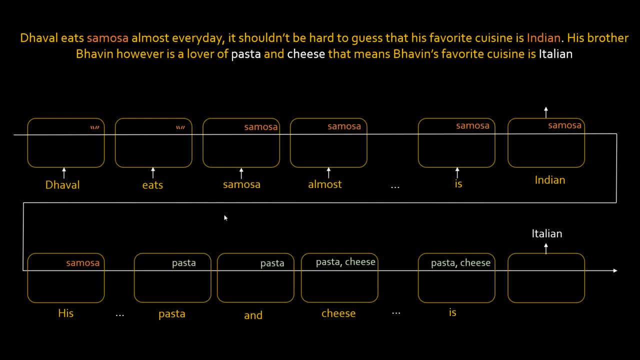 all of this happens during the training process. so when you're training your RNN, you are not giving only this particular statement. this is this is a statement for prediction. when the training is happening, you are giving thousands and thousands of such statements which will build that understanding in RNN on what 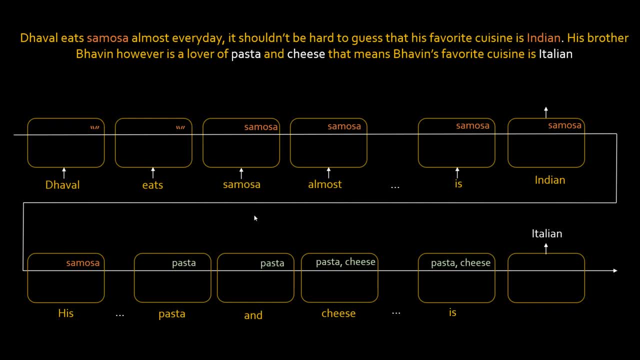 to discard and what to store. so here we learnt a very important concept, okay, so when you're talking about LSTM, or a long, short term memory cell, so each of these cells are LSTM cells. the first, most important thing is the forget get. so the role of forget get is, when you come at this word, pasta it. 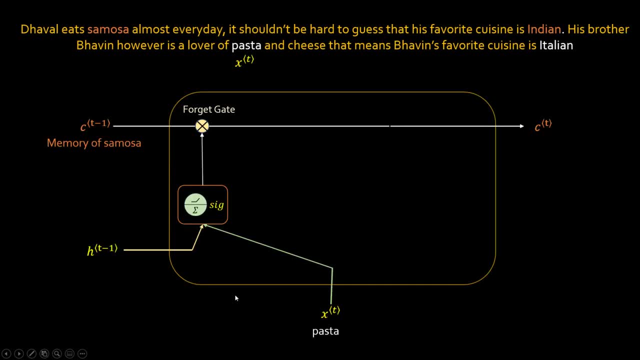 knows that it has to discard samosa. okay. so this is how forget get looks like. so I have just expanded that cell. xt is a one word. you know you process sentence one word by one word and t is the timestamp, so that's why xt. so when you feed pasta into this, forget get. so the forget get is: 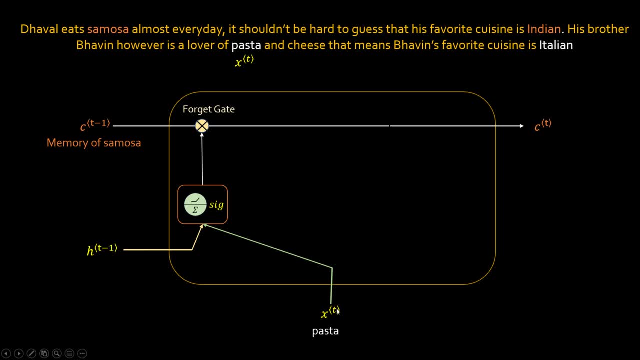 simple. you have previous hidden state, you take the current input, which is a current word, and you apply sigmoid function. now you know that sigmoid function or restricts your number between 0 and 1, so it will. if it has to discard the previous memory, it will output a vector which will have all. 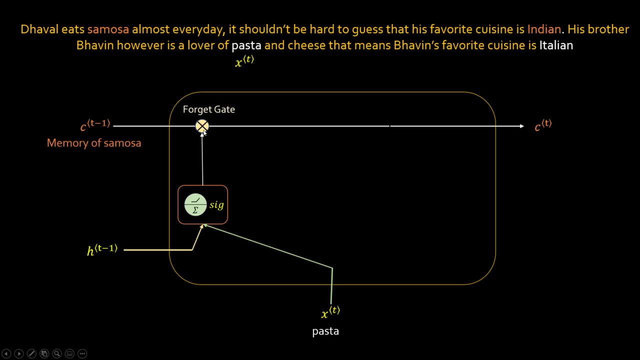 zeros or all the values which are close to 0. and when you multiply that with previous memory, which is previous cell state, you know you have a vector of, let's say, all zeros here and you have another vector which is a memory of previous cell state. the multiplication will of course be 0, because you have 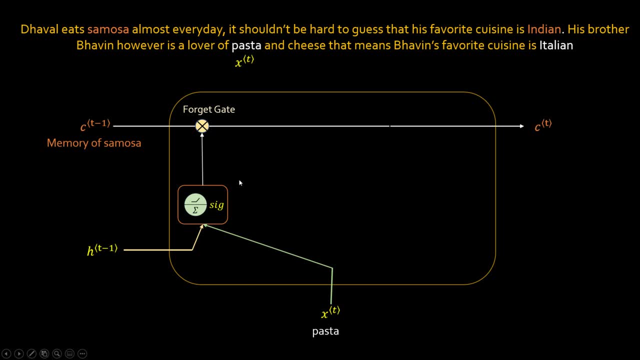 discarded the previous memory. you know when this new word appeared, so this is what a forget get looks like. so here, you forgot about samosa. now there is another thing, which is an input gate. so when pasta came, not only you forgot about samosa, you need to add a memory of pasta. so the way it will work is you. 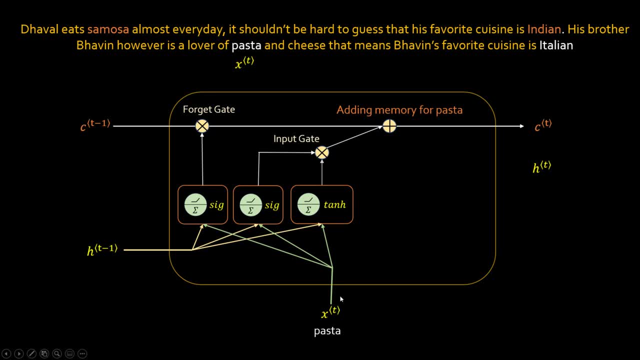 will use sigmoid and tanh both on these two vectors. okay, so when you're doing, by the way, these vectors will have weights here, so there will be some weight here, some weight here. so in this function what you're doing is H? T minus 1 into that weight, plus X T into that weight plus bias, and then you're. 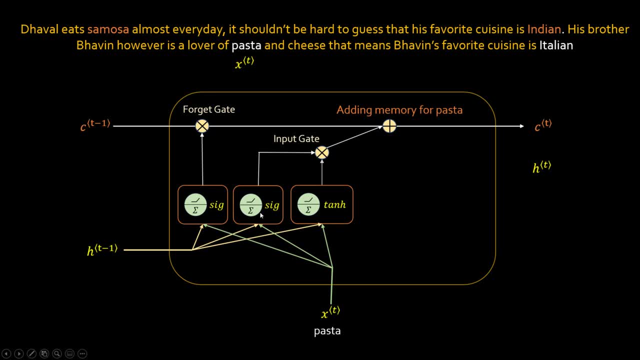 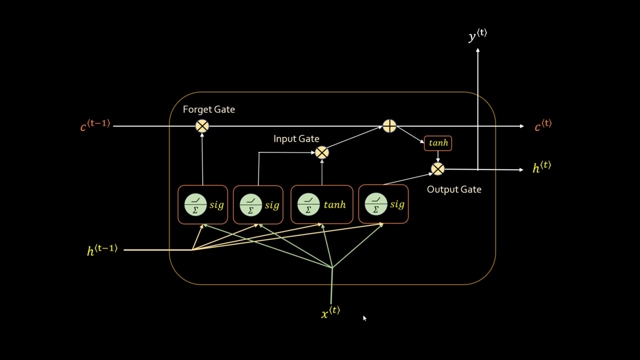 applying tanh on top of it. and it's the same equation here. the only difference is, instead of tanh you are using sigmoid function and you multiply both of this output and then add that as a memory for this word. the third one is output gate. so in the output gate again you are doing weighted sum of hidden state and 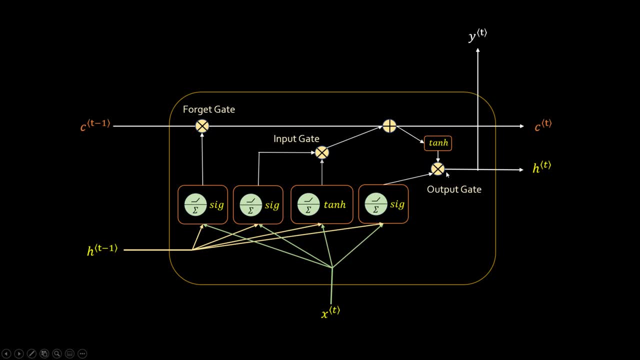 X, T and applying sigmoid function, whatever is the output, you take that and then you take long term memory, apply tanh and you multiply that and you will get your hidden state. okay, so this will be your hidden state. there are cases like Lang- let's say the sentence autocomplete case that we were looking at. 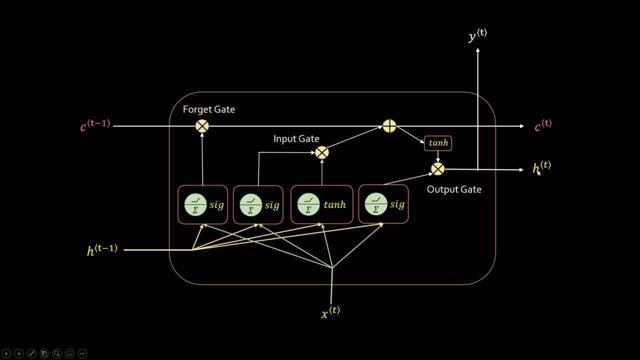 yt. actually the state is carried using the short term memory. but you know, if there is a task like a named entity recognition, there you need yt, which is an output, and that output is same as H? T. I mean you might apply sigmoid, not sigmoid but let's say softmax type of function here. but other than that it is. 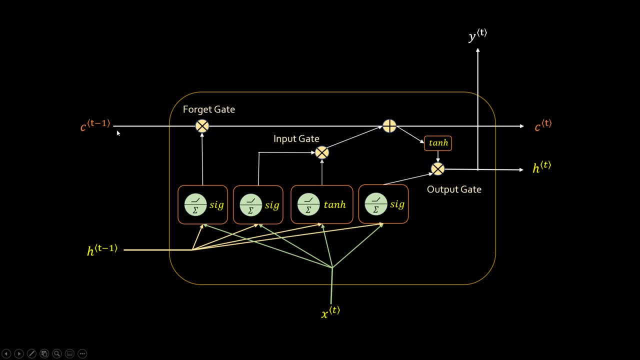 kind of similar to H T. so now, if you think about the long term memory, so long term memory, look at this line. okay, look at this highway, for example. it has two things: forget gate and input gate. so forget gate is like it will help you forget things like samosa when pasta comes in, and the input gate will add new